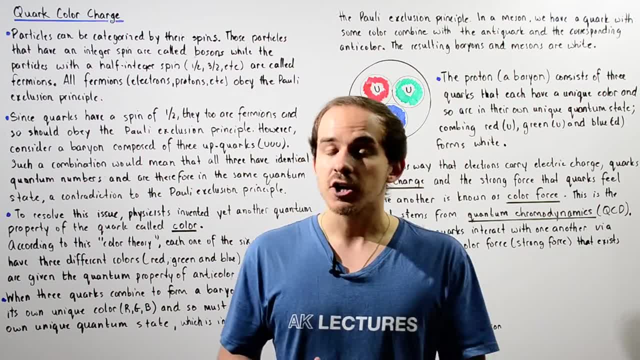 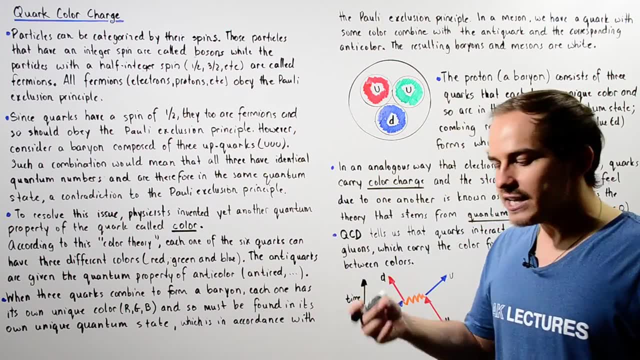 the Pauli exclusion principle. However, fermions must obey the Pauli exclusion principle. Now, the bosons do not need to obey the Pauli exclusion principle, However. for example, the electron is one example of a fermion. The electron can have a spin of. 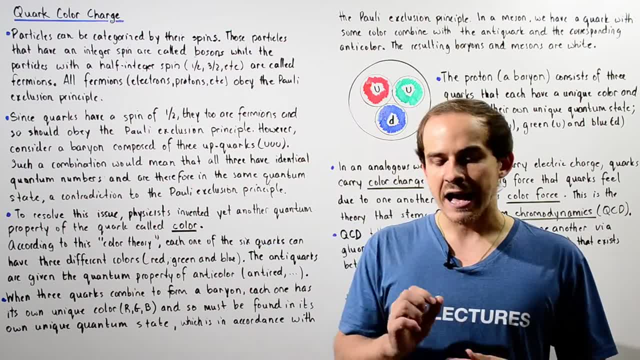 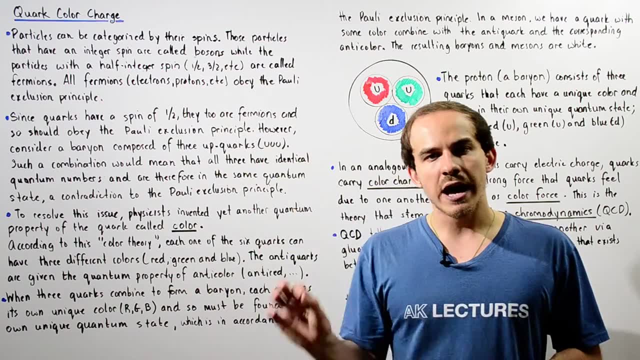 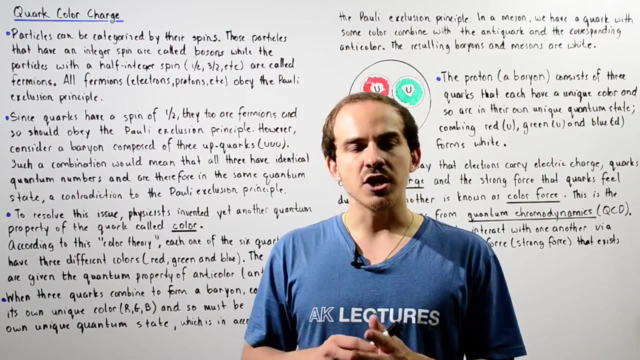 negative, one half, or a positive one half spin. And we know that whenever we have an electron in any given atom, that electron has its own unique quantum state that is designated by the various types of quantum numbers. Now a quirk is also considered. 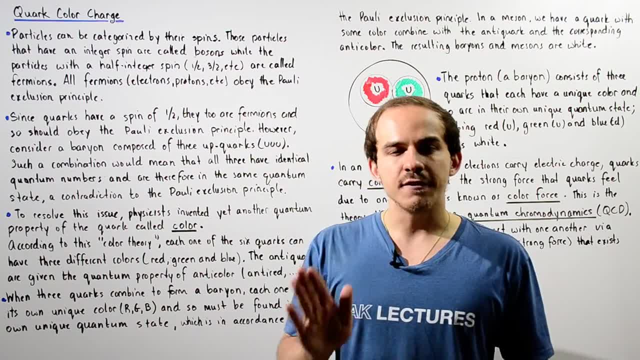 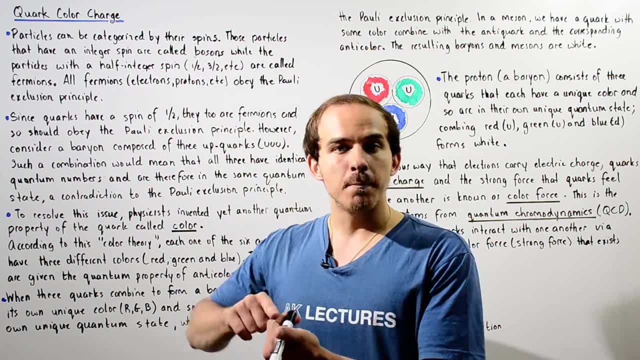 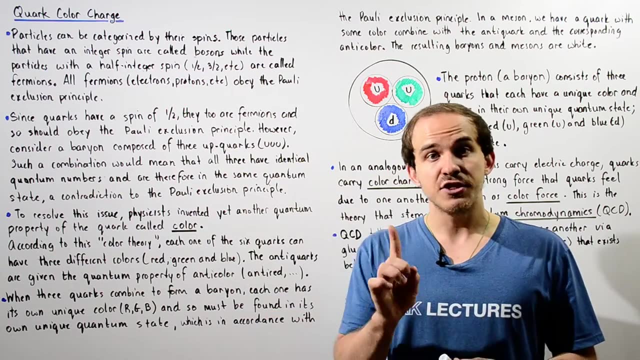 a fermion, because all the six different types of quirks have a spin of one half. So the up and the down, the top and the bottom and the strange and the charm quirks, all these quirks have a spin of positive one half, And that means, by definition, the quirks are fermions, And so 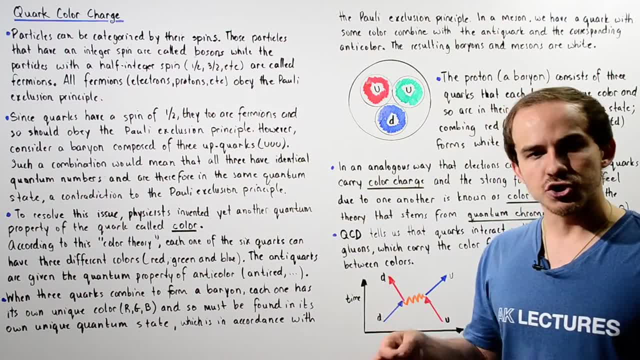 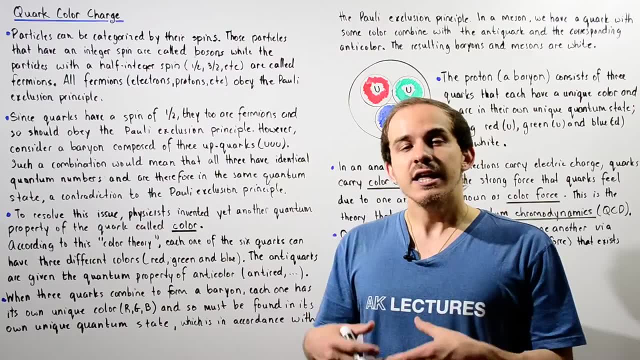 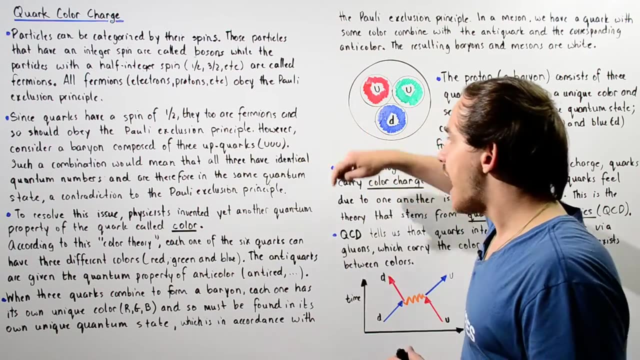 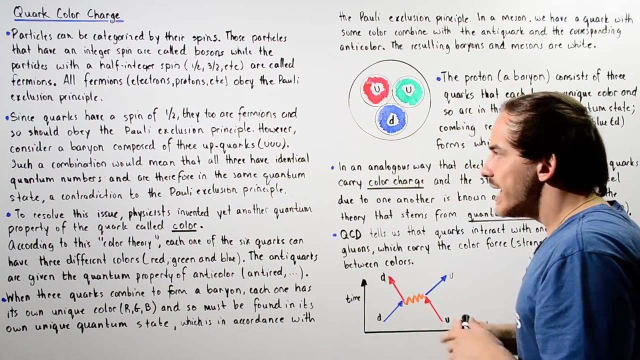 they must obey the Pauli exclusion principle. However, let's suppose we we have a baryon, a baryon that consists of three quirks, And these three quirks are all up quirks. So we have U, U and a, U that basically compose the baryon particle. Now, each one, 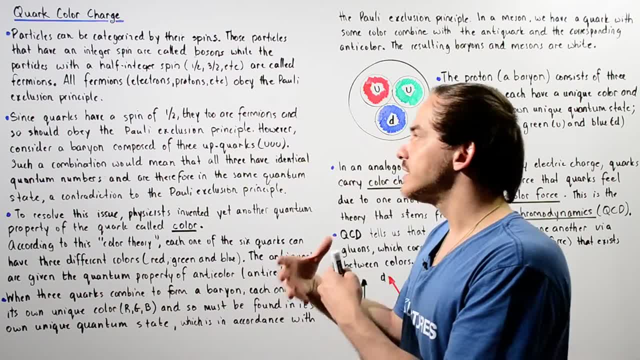 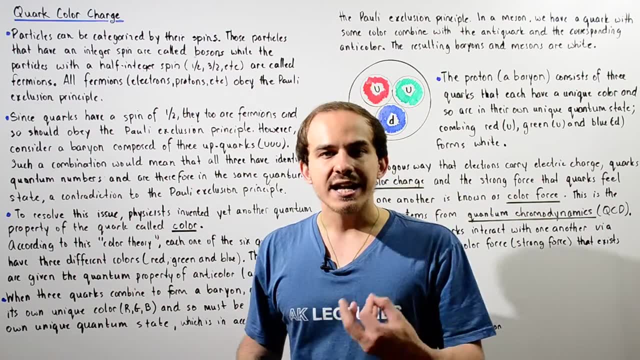 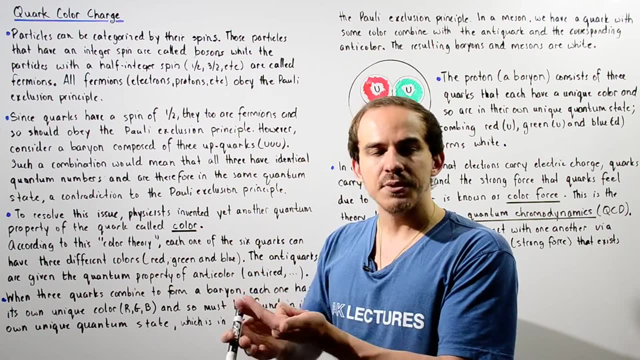 of these up quirks has its own quantum numbers. Now, all these U's have the same exact quantum numbers. We know that any up quirk has its own quantum numbers. Now, all these U's have the same charm. quantum number has the same strangeness, has the same topness, bottomness. 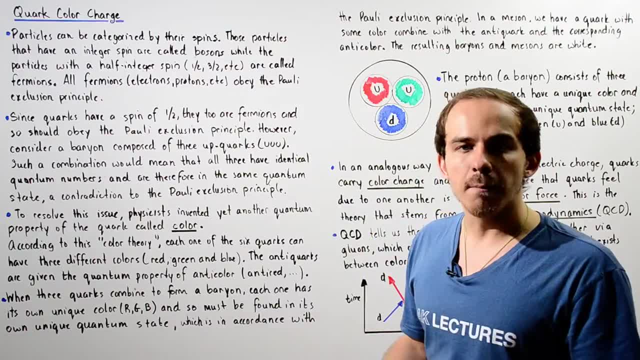 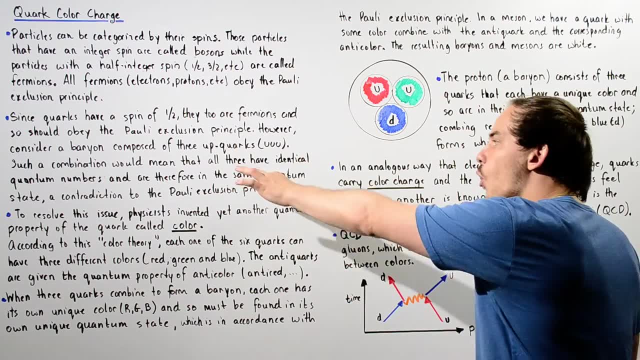 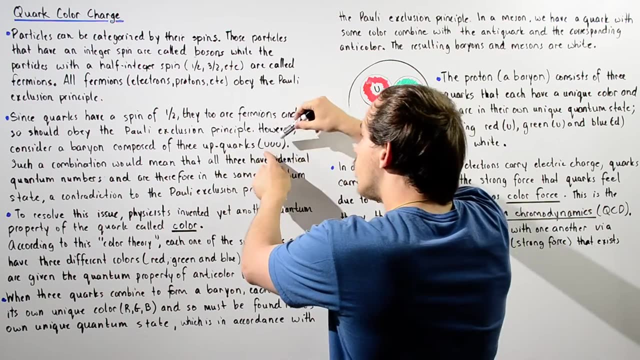 has the same spin, has the same lepton numbers, baryon numbers and so on, And such a combination would mean that all the three quantum numbers are exactly I. I mean all the quantum numbers for all these three up quirks are exactly the same. And that basically means that 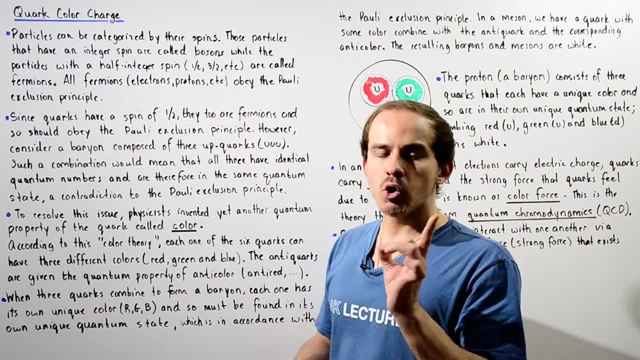 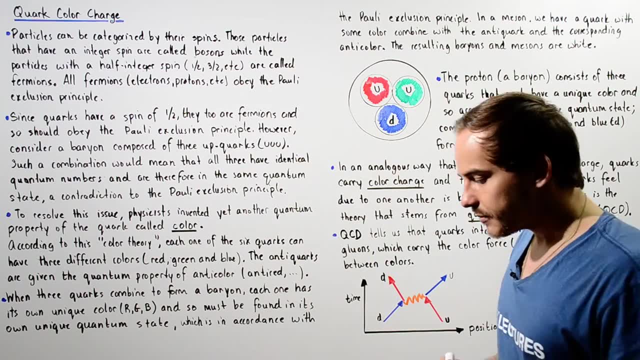 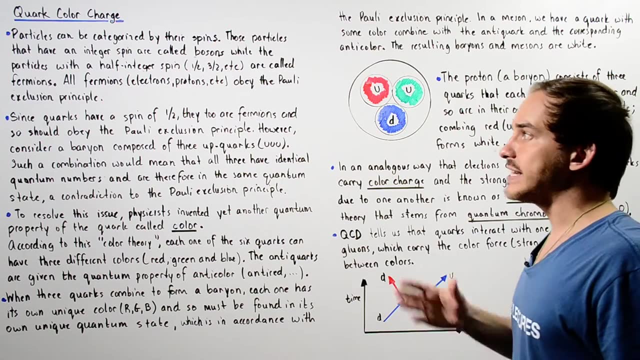 that they must be found in the same exact quantum state, which is a contradiction to the Pauli exclusion principle. Now, to resolve this issue about quirks being fermions and not obeying the Pauli exclusion principle, physicists came up with another quantum number. 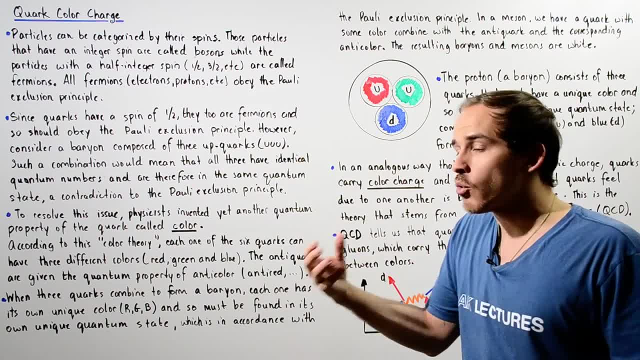 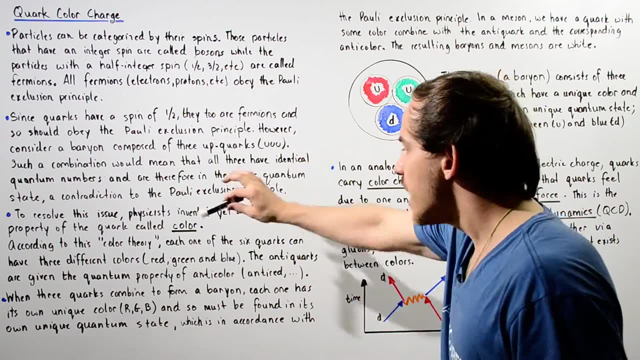 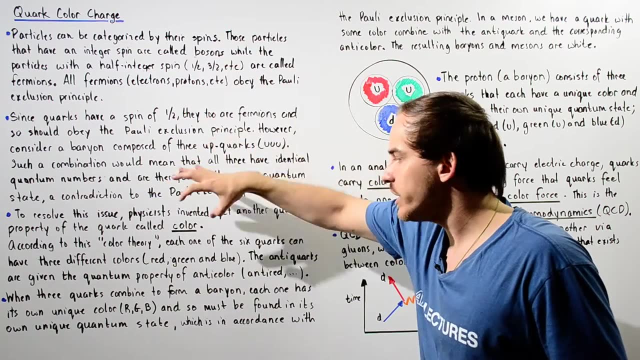 So they say that quirks have yet another quantum property that we call color. So, baryon, quirk means quirk. So, based on this color theory of quirks, each one of the six quirks can have three different colors. So we can have red, green and blue. Now the anti-quirks. 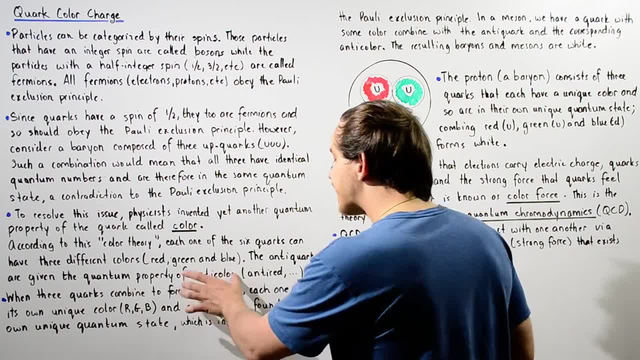 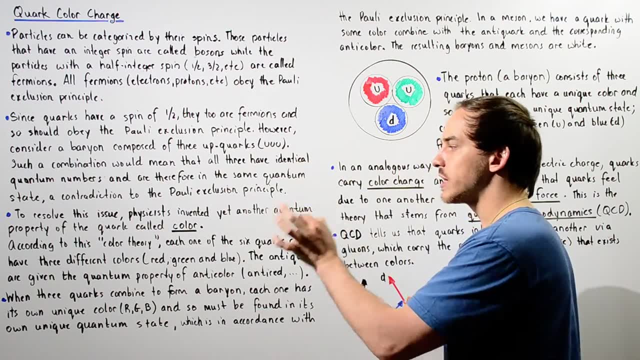 are given the quantum property of anti-color, So anti-red, anti-green and anti-blue. For example, if the up quirk has the red color, the anti or the up anti quirk will have the red color and the up level quirk- the first one has the. that means a gold color. OK. now the anti-reahaha bet types also theeumachen the peersơn, AKA Dutch, saying that quirk is a rare Argentine. quirk bello VAEAVA, whar ae and other. these three come from a lot of. 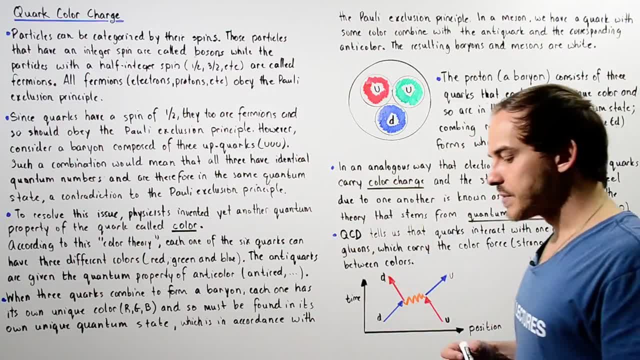 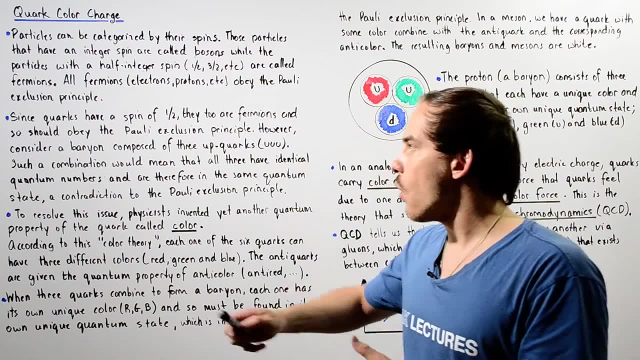 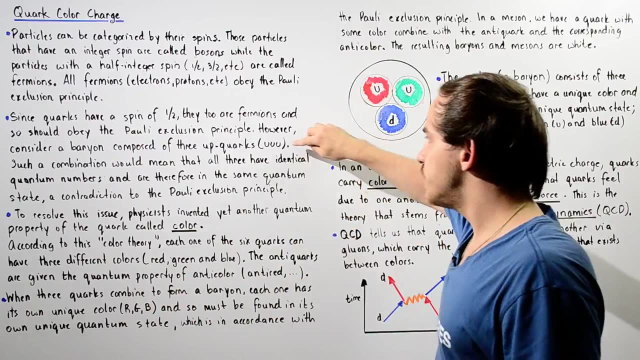 other characteristics that work. And the elite, L' üst, jumps out when the alfazhe-sam outfits have the anti-red, anti-color. So this basically means that when we take three quirks and we combine them to form our baryon, each one of those quirks has its own unique color. So in this case, 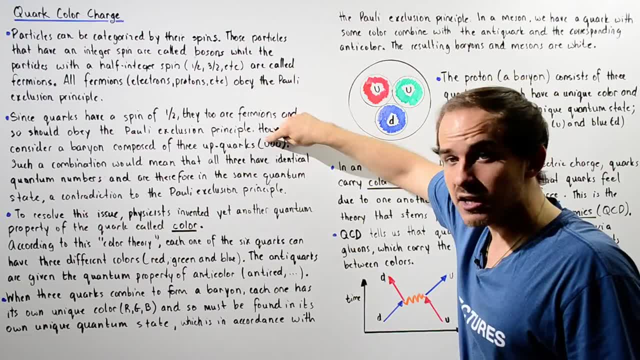 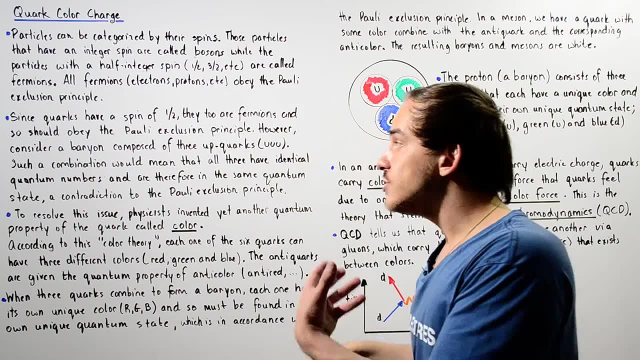 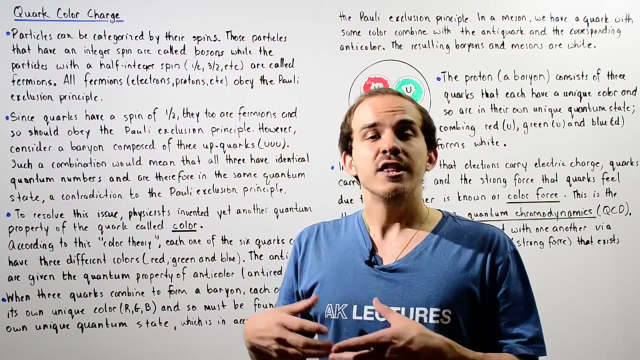 the first U, the first up quirk, would have the red color, the second one would have the green color and the third one would have the blue color. And because each one of them have their own unique quantum number called color, that means they are all found in their own unique quantum state. 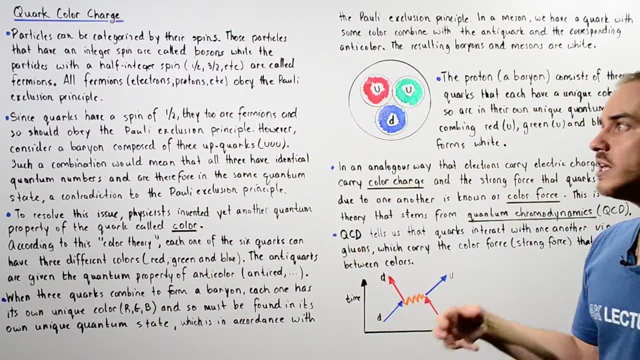 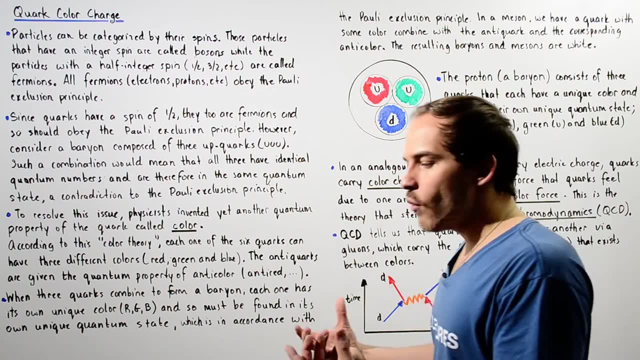 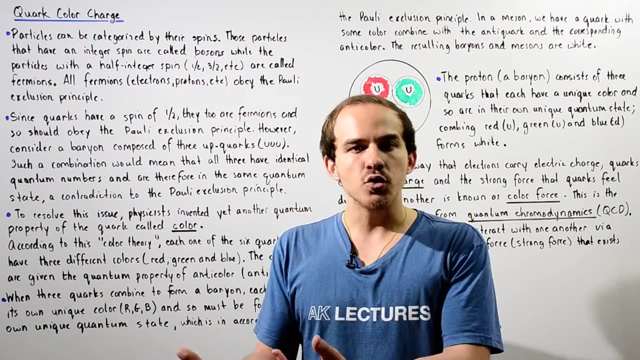 And that means that quirks readily obey the Pauli exclusion principle. Now, in the same exact way, we can also form a nascent from a quirk and an anti-red, And in such a case let's suppose we're using our up quirk and we want to combine that quirk. 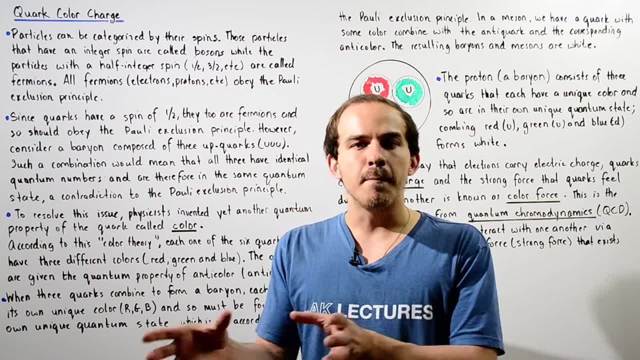 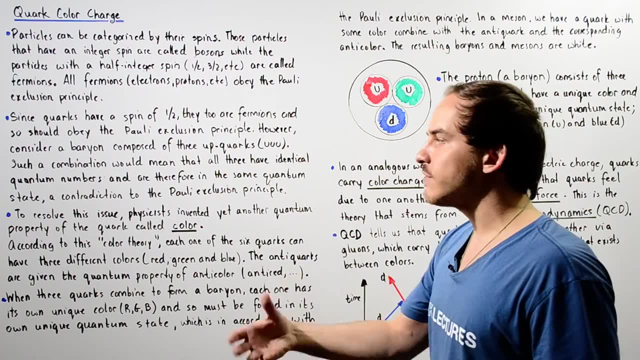 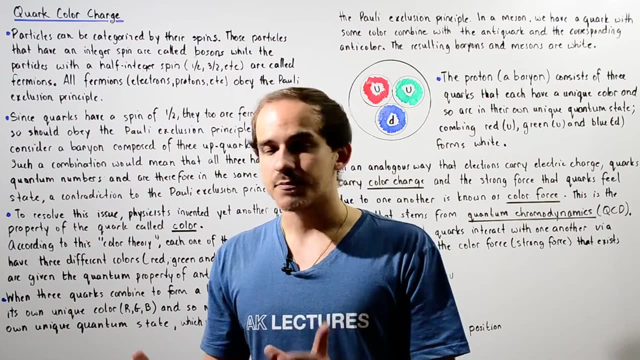 with some anti-quirk. So we're basically combining a color and an anti-color. Now, whenever we form baryons and whenever we form nascent, the actual color of those baryons and nascent is white. So, for example, let's suppose we have the following baryon: 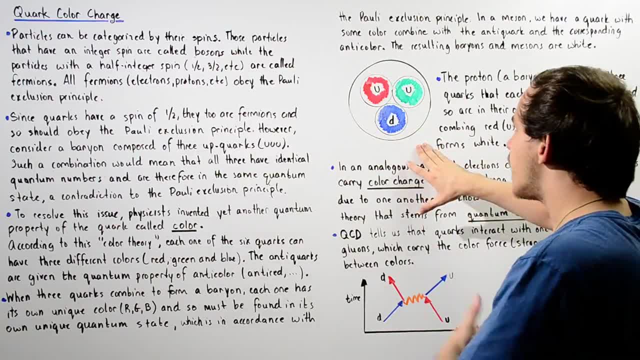 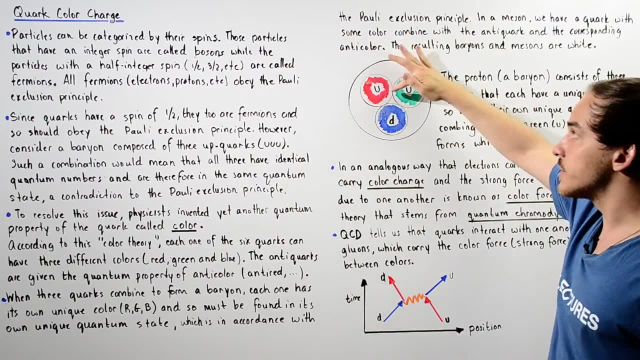 This is a proton. A proton consists of the up quirk, the up quirk and the down quirk. Now, in this case, the up quirk, the first up quirk, has the color red, and that means this must have a different color. 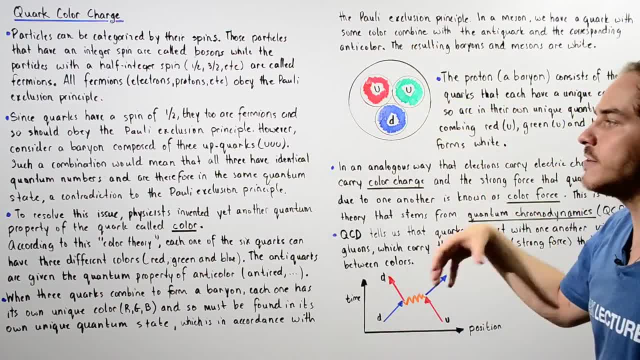 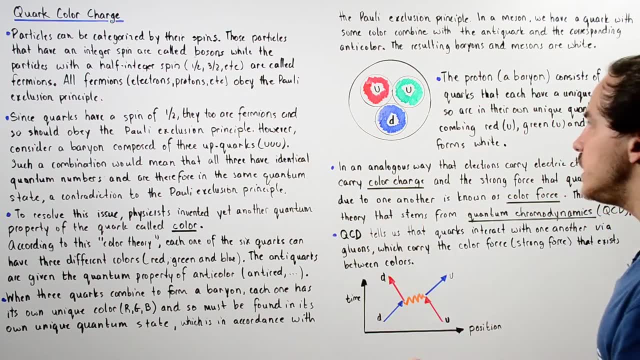 We're going to say green and the down quirk must have the final color, blue. So this means each one of these is found in its own unique quantum state and this is in its own unique quantum state, And this is in its own unique quantum state. 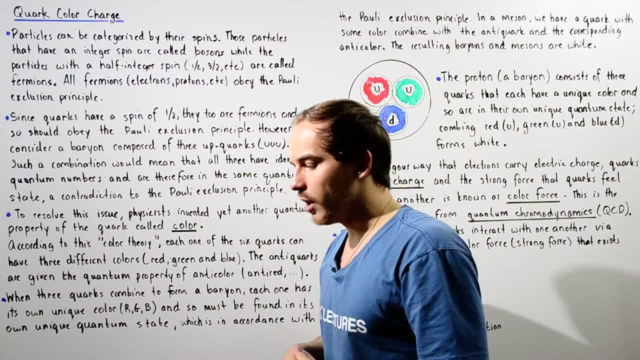 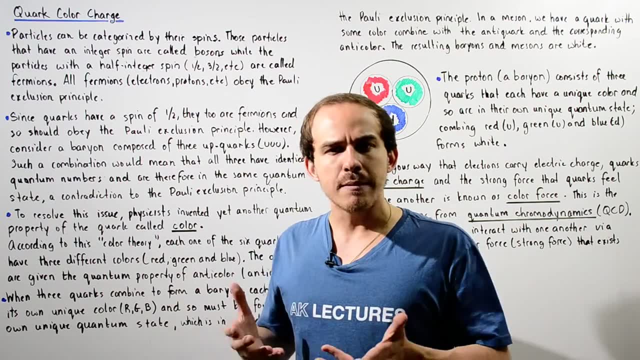 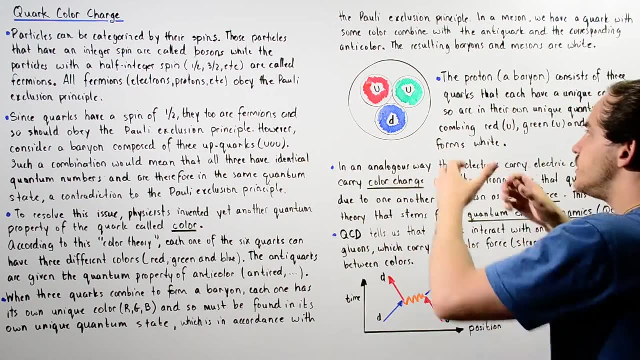 And this is in its own unique quantum state, In accordance with the Pauli exclusion principle. Now we know that whenever we combine the color red, blue and green- these are the three primary colors- we form the color white, And that's exactly why we say the proton is the color white. 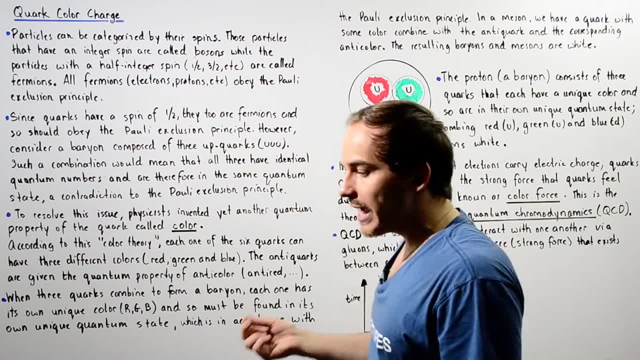 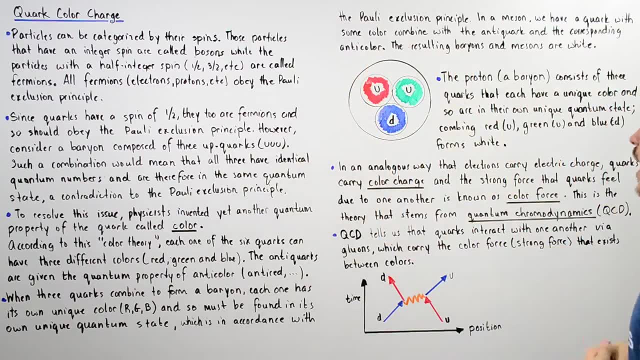 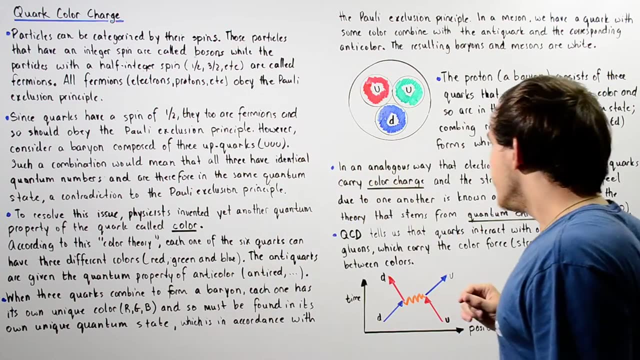 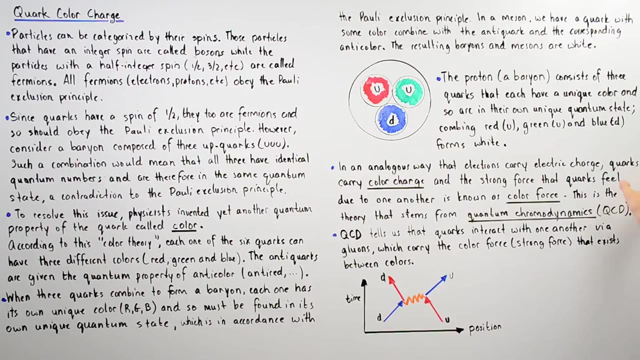 The proton as a whole has the color white because when these three quirks combine, we combine red, Green and blue, and that forms white. In the same analogous way, mesons also form white colors. Now, in an analogous way that electrons are said to carry electric charge. 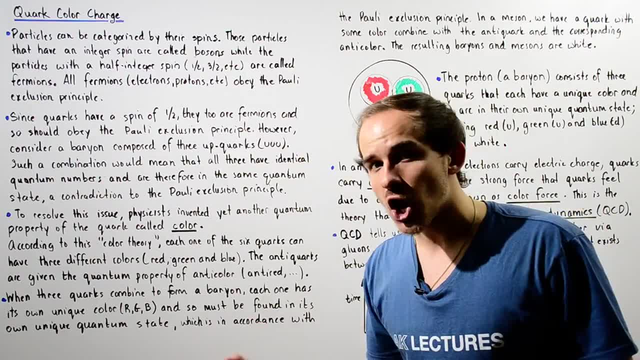 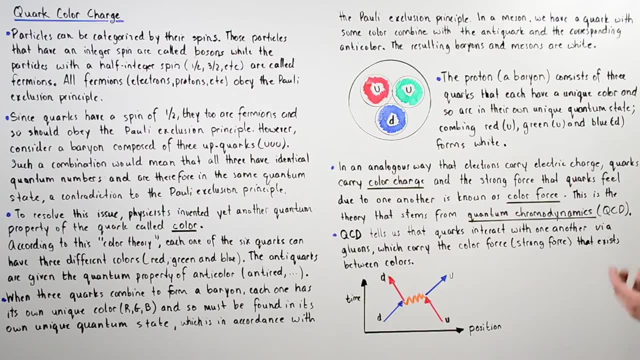 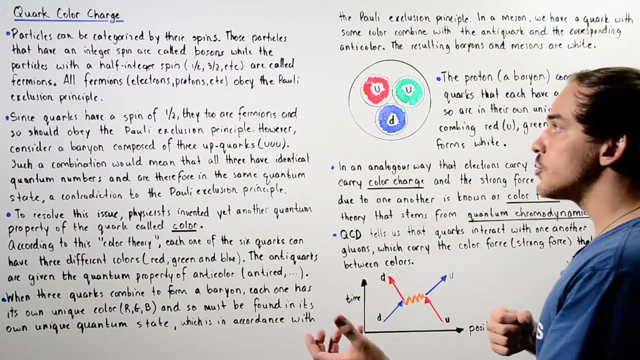 quirks carry something called color charge, So each one of these colors produces its own color charge and the strong force, the strong nuclear force that makes them force, that quarks feel due to one another, between one another, is said to be the color force. So in 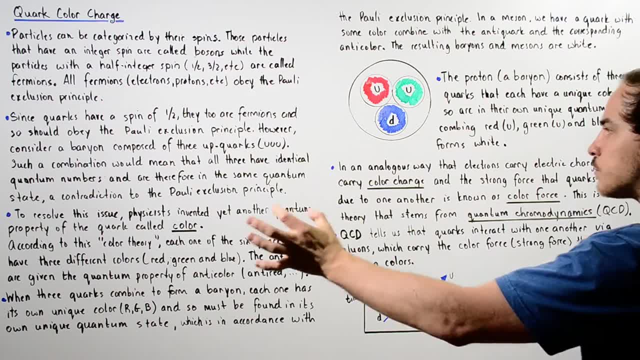 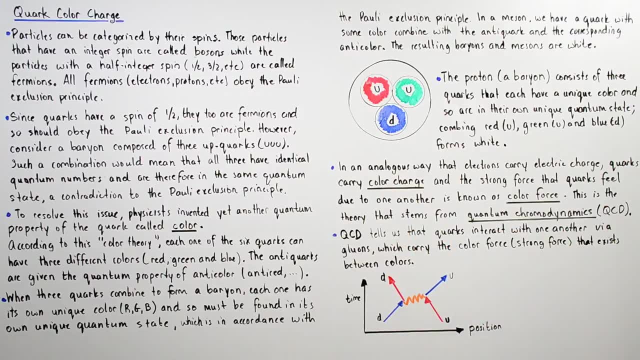 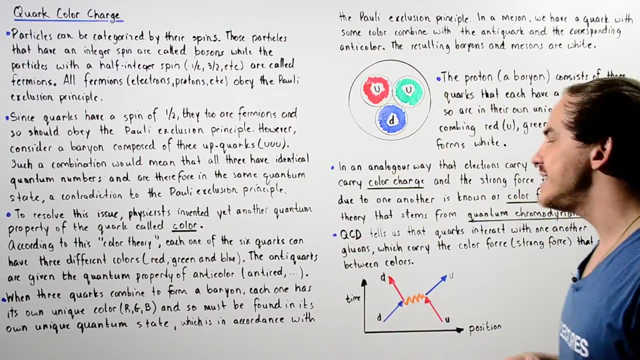 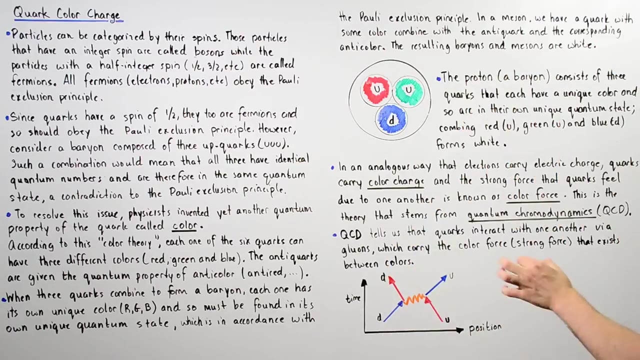 the same way that electric charge is said to produce the electromagnetic force, the colors have color charge that produce the color force. Now this idea comes from the field known as quantum chromodynamics or QCD. Now, quantum chromodynamics tells us that quarks interact. 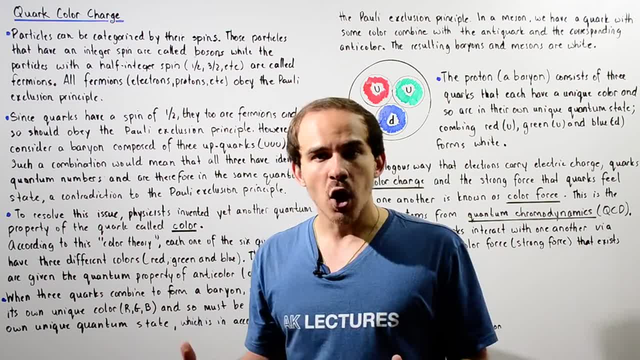 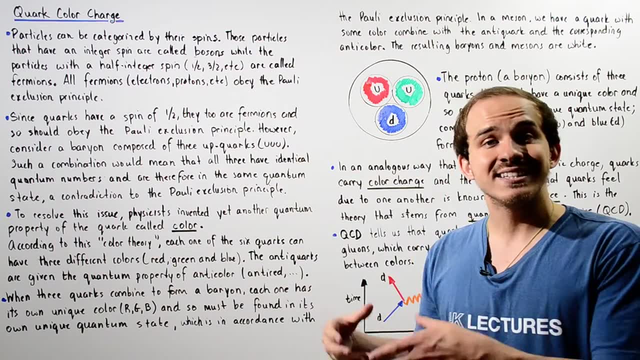 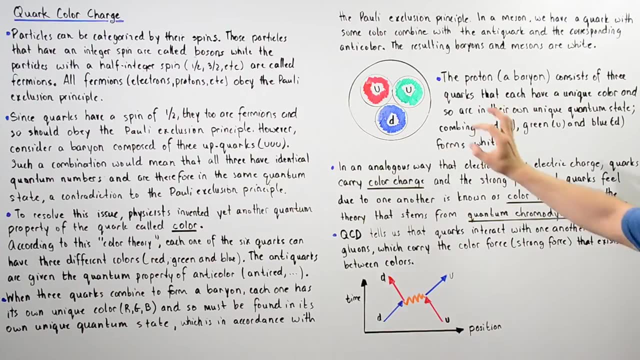 with one another via gauge bosons, fundamental particles known as gluons, And these gluons are said to carry this strong nuclear force. we also call the color force that exists between the different colors on our quarks. So this Feynman diagram describes the way that our down quarks with the blue color and 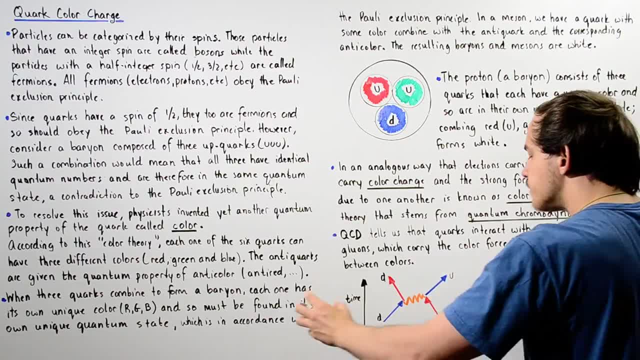 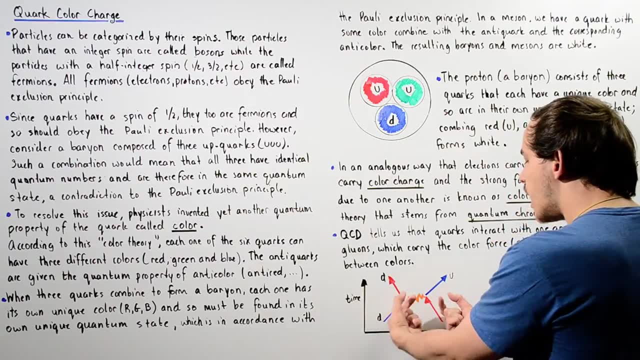 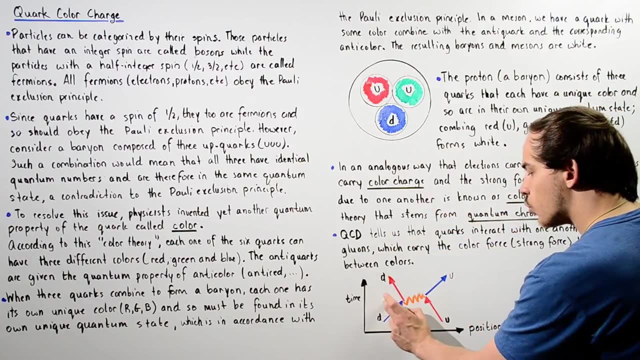 the up quarks that has the red color interact with one another. So, basically, as these two quarks approach one another, when they get close enough, our quarks releasing the gluon and the quarks getting closer to each otherして at the eventually, puedo ser USA ν. Our one of these quarks. lets say this quark releases the glue ion and the zelonionnen quarks on the opposite of our quantum chromem오너로. 자세한 과정 complete will be generated by getting these two quarks to interact each other usingquadron. So to responding. 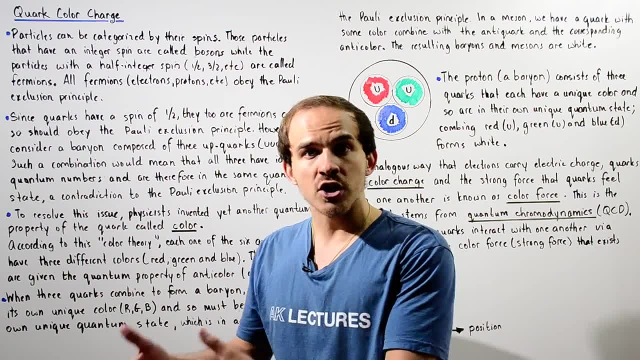 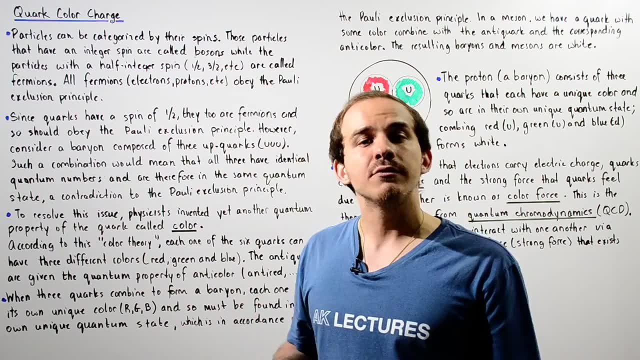 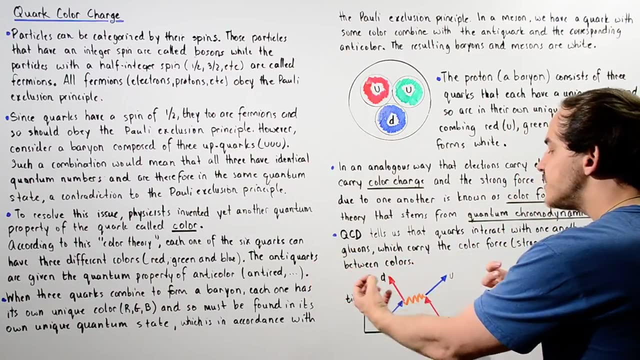 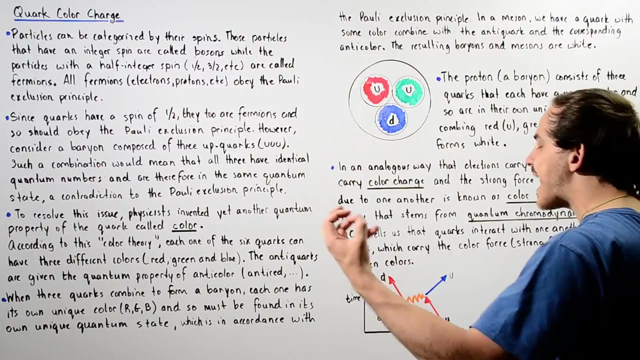 this gluon carries this strong nuclear force we call the color force, And when it carries this color force, it also carries the color of this particular quark, And so that's exactly why we have an exchange of color. So this down quark used to be blue, but when it released that gluon, 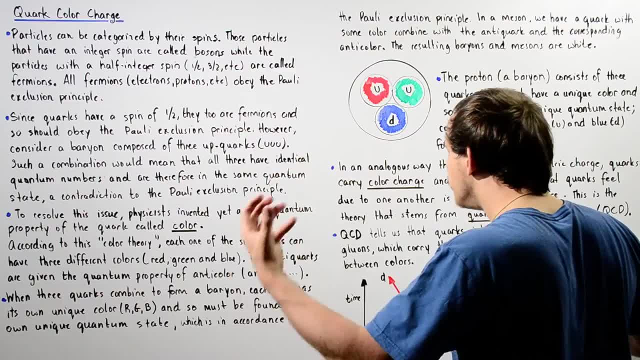 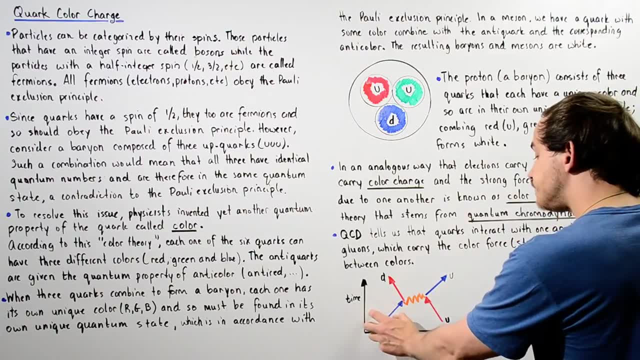 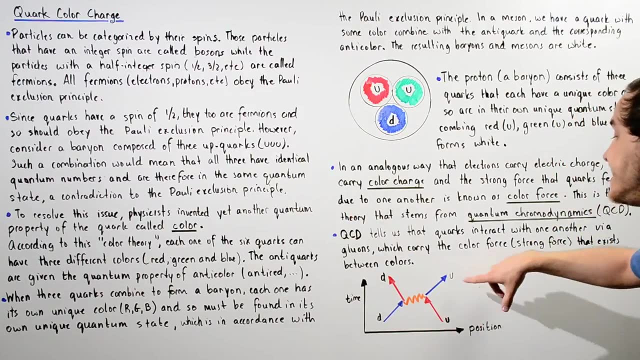 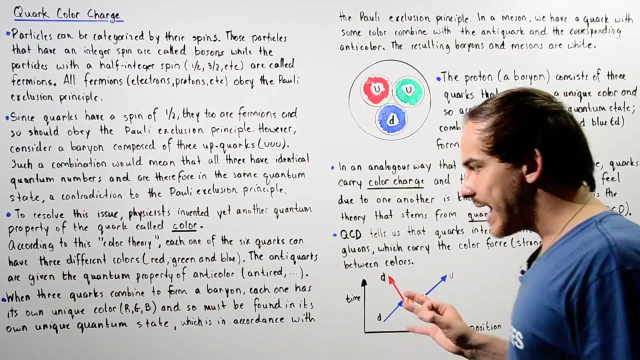 that gluon basically released that blue color And basically they exchanged the colors. So this D, this down quark, which was blue, now becomes red, And this up quark, which was red, now becomes blue, as shown by this Feynman diagram. So once again, basically every single quark. has a different color. 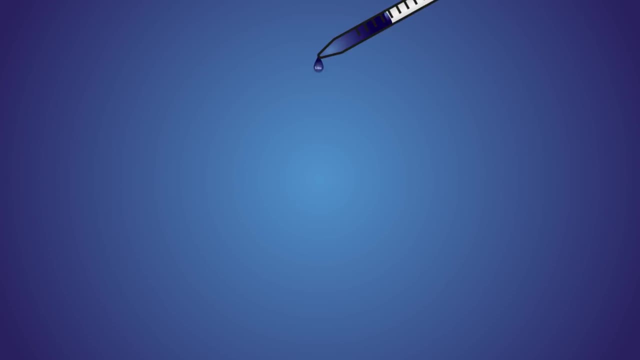 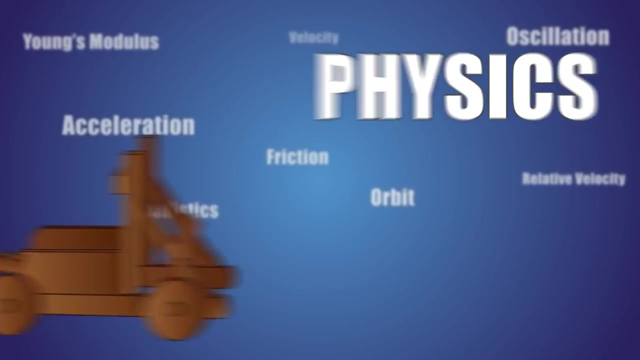 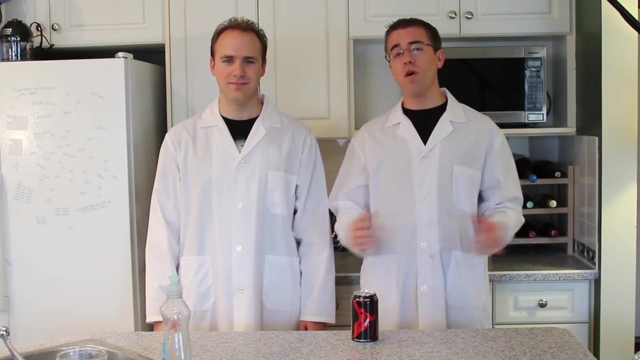 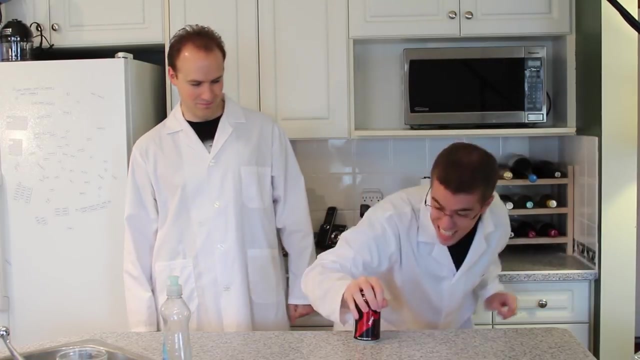 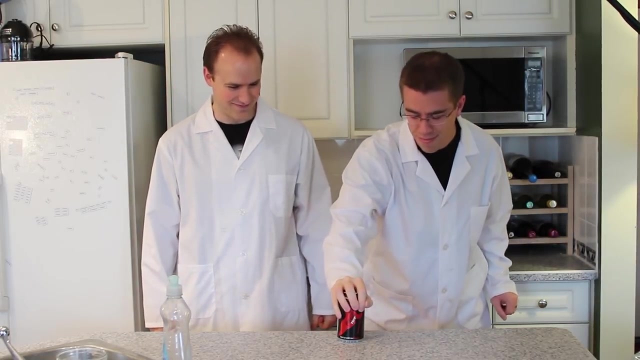 Today on Sci Guys can crush. Welcome to Sci Guys. I'm Ryan, I'm Adam. On today's episode we're going to be crushing cans using air pressure. I'm going to crush something. It's supposed to be open. Yeah, I guess you're right.